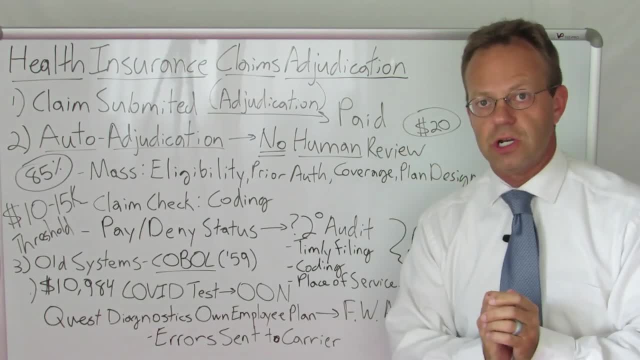 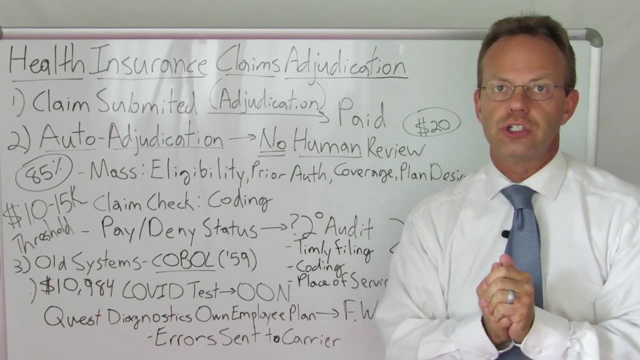 Okay, so the process of auto adjudication has several parts that we're going to go over. There's a fantastic slide presentation By Aetna to doctors and hospitals themselves that I'll leave a link to in the show notes, because they're explaining how the adjudication process works. 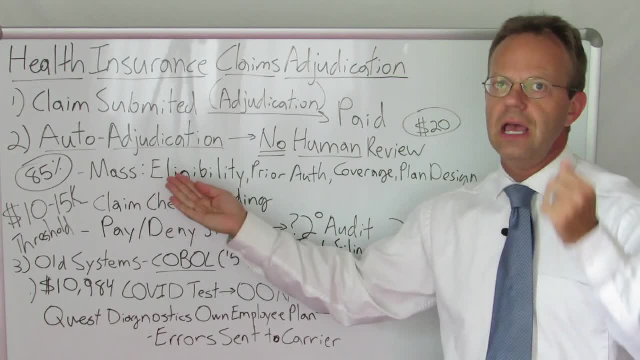 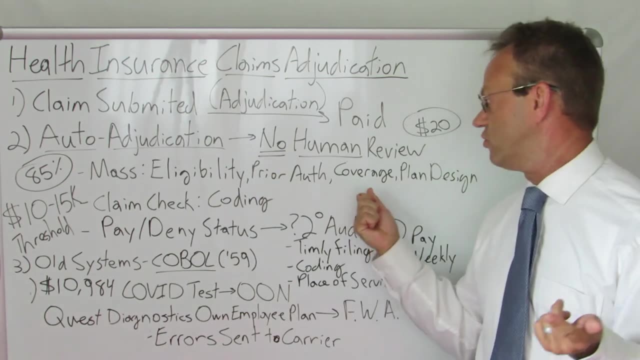 So you start with mass adjudication, where the software looks for things like eligibility of the patient. They look for if any prior authorization was needed to process the claim. They look to see if it's for a covered service or not. They look to see if the plan is designed to see if it's going to be deductible or copay or coinsurance, etc. 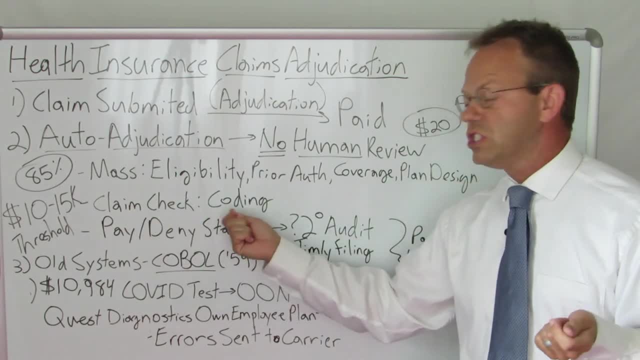 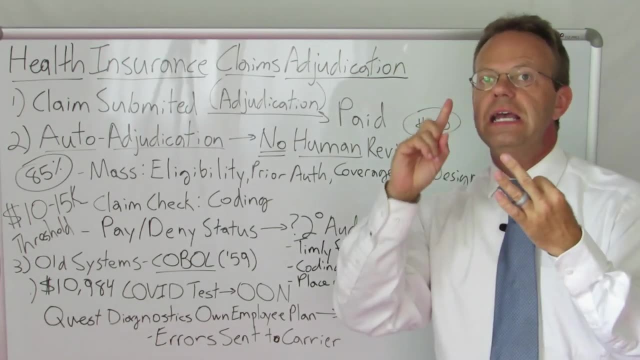 Next, it goes through a claim check, Which is where the actual cost is. They look at the codes on the claim, In other words the ICD-10,. if it's an inpatient code, then it's the DRG. it's looking at the CPT codes. it's looking at the HCPCS codes. 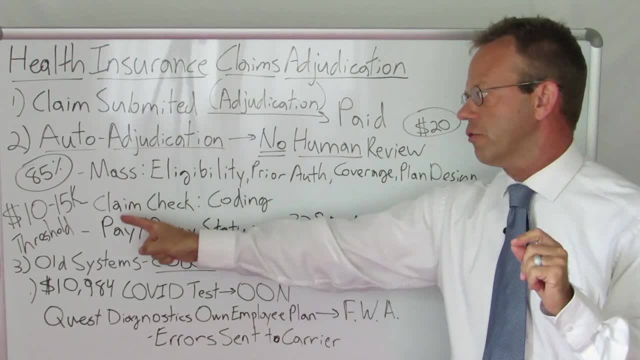 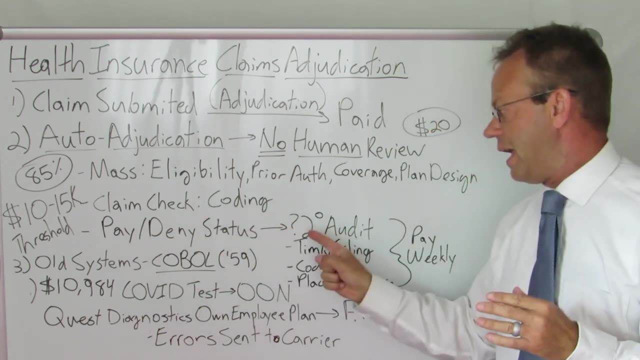 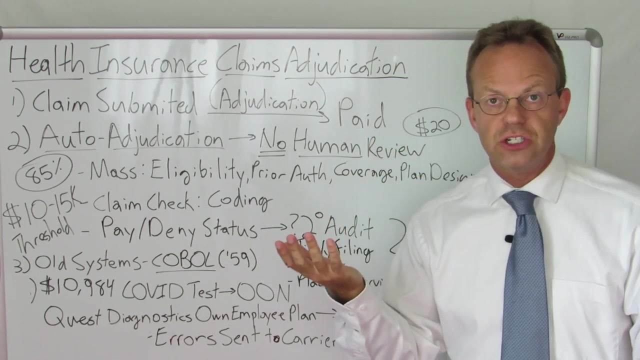 That's when the actual codes get examined. It's done during this claim check And then it moves to either pay or deny status, And if it's in pay status, then it's going to get a secondary audit. Now, as you can understand, the entire adjudication process is proprietary to the insurance company. 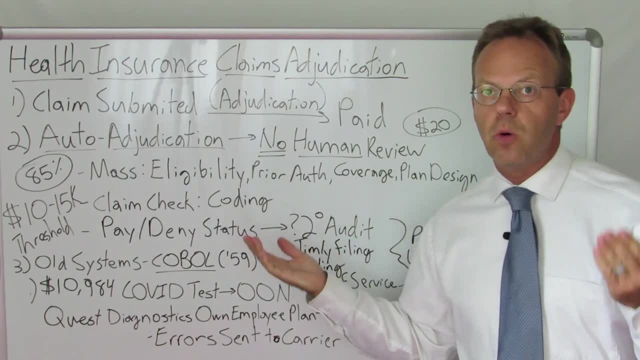 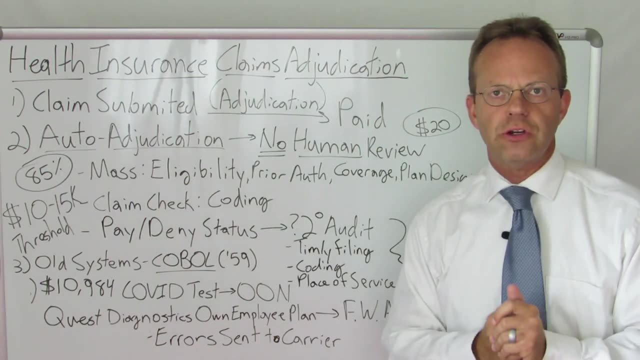 So there's only so much that they're going to tell about this, But in the quote unquote secondary auditing process they're going to check for timely filing requirements. In other words, oftentimes you can't just submit a claim two years after you saw the patient. 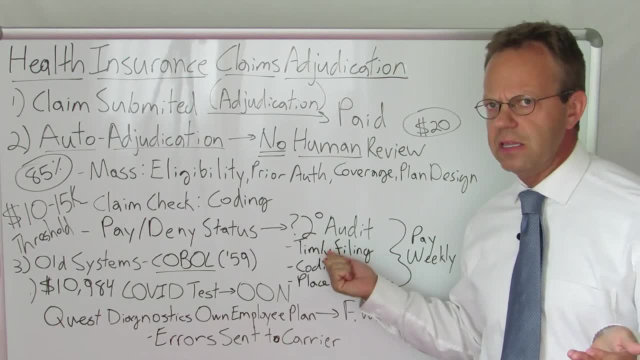 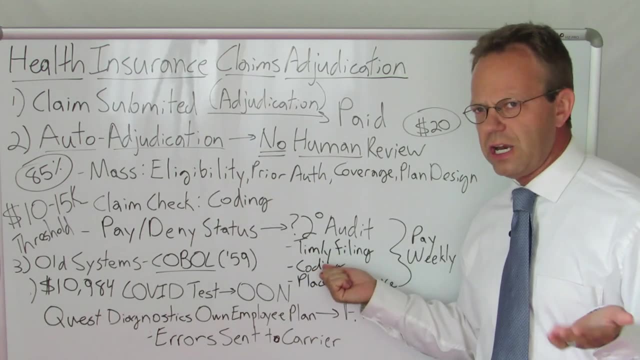 Which begs the question: why in the world would they sync timely filing requirements to the end? Why don't they put it at the beginning? That doesn't make any sense. Next up again, they look at the coding again. Well, what in the world are they going to look at in the coding in the secondary audit that they could have just looked at on the coding upfront? 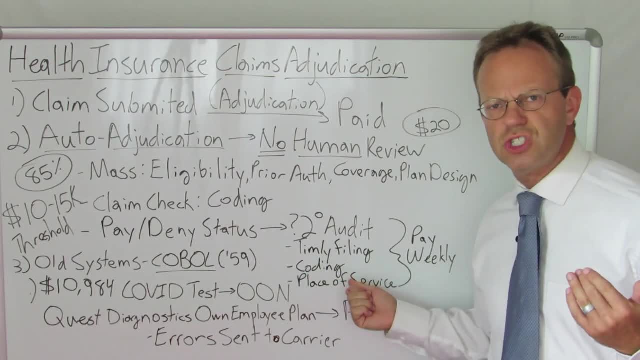 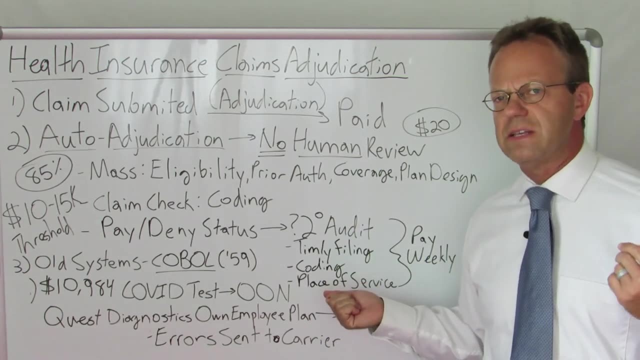 That doesn't really make a lot of sense. And then they're going to look at the place of service, What to determine, like the provider tax ID, to see if it needs to be processed in or out of network, Or to see if something is being done inpatient that could have been done outpatient. 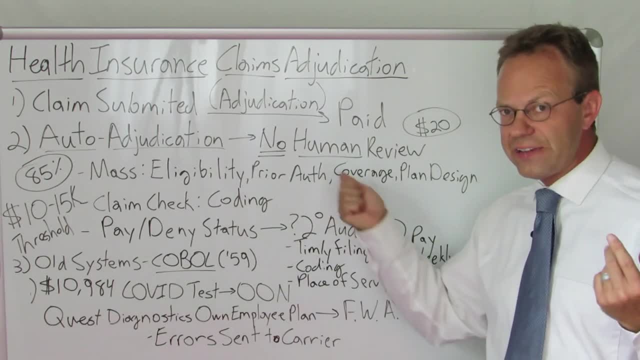 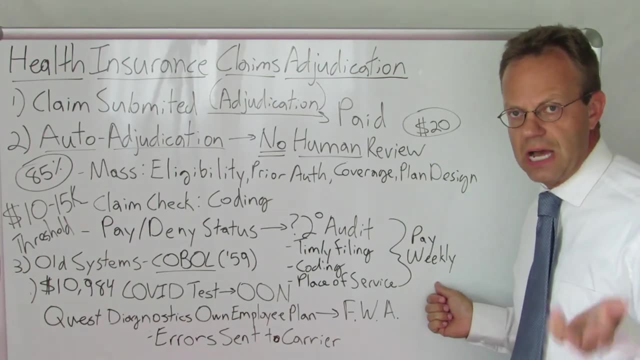 Again, it seems kind of odd that they're putting it here and not earlier on. And then, if it gets through that process, then they pay out weekly, Typically by electronic transfer to the bank account to the doctor or the hospital. Okay, fine, Here's some problems with auto adjudication. 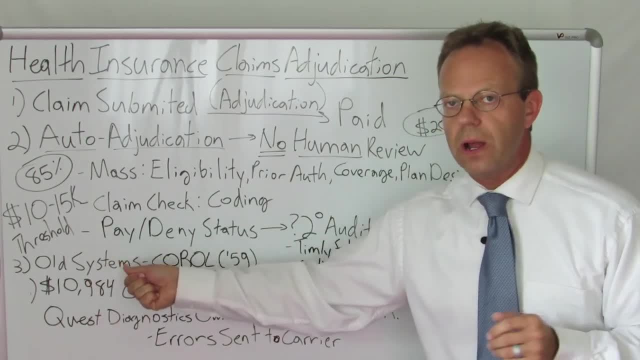 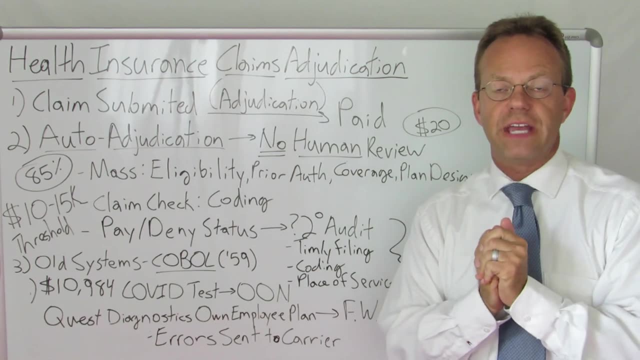 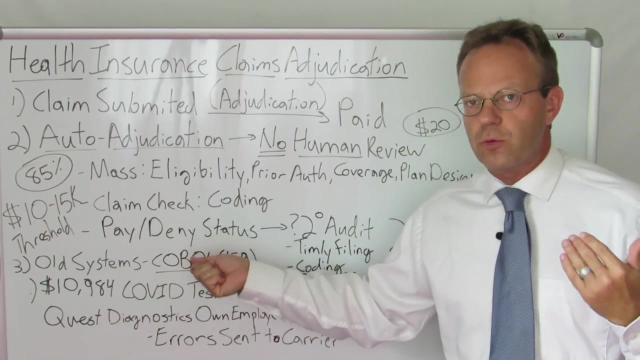 Is that it's written in very old software. I was speaking to a former examiner. He was an executive from an, And a lot of insurance carriers actually outsource claims adjudication to third-party companies where all they do is adjudicate claims, And a lot of that software is still in COBOL, which is a software language that was originally created in 1959.. 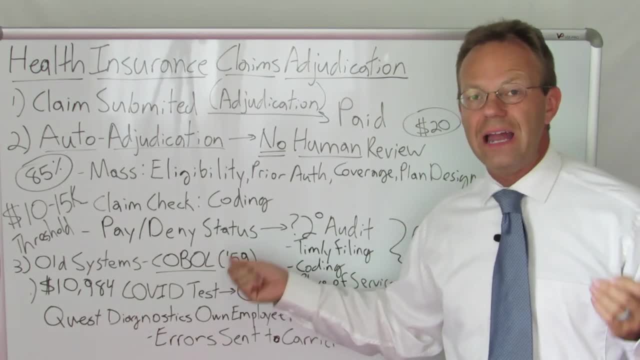 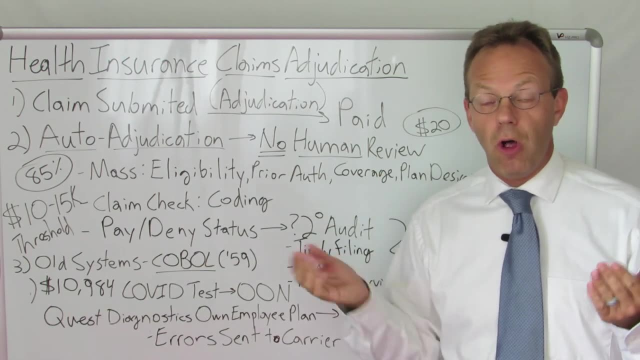 COBOL is an acronym. The software was created in 1959.. The problem with COBOL is that the number of programmers- because it's so old, the number of programmers who actually have expertise in COBOL- is small And it's getting smaller because they're retiring. 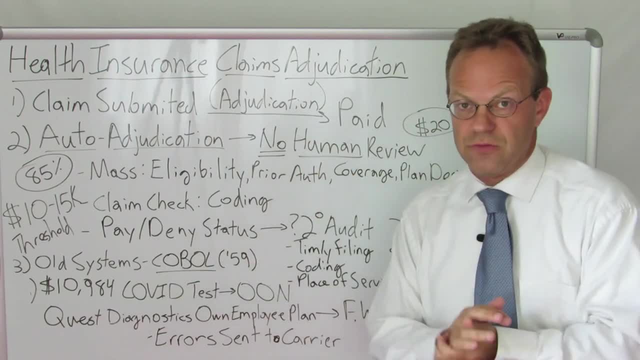 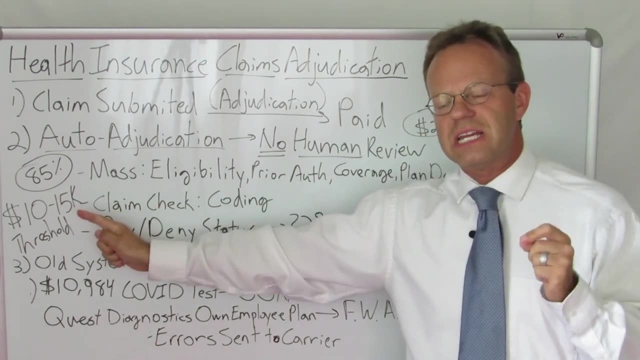 So there's just not as many people around who actually understand it. They don't understand the COBOL language very well And then typically because this process is so expensive if you do it manually, oftentimes the carriers will set dollar thresholds on the claims, where they just let it pass through. 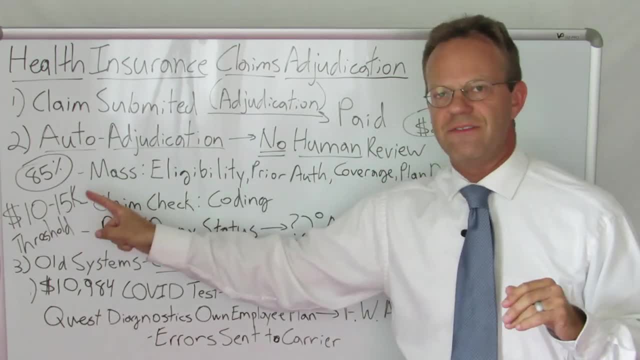 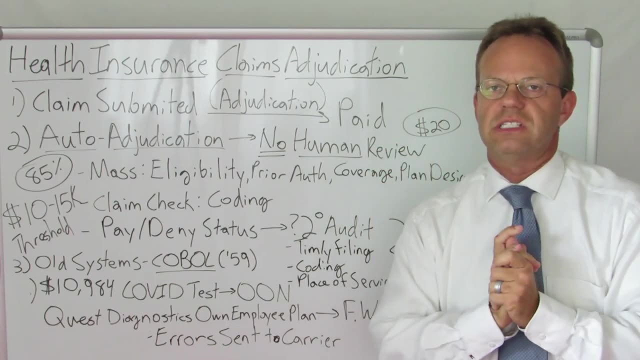 And they're not going to have any manual review for claims of less than $10,000 to $15,000.. Okay, So what are the consequences of this? What are the real-world consequences of this for individual patients and the plan? So there was just a story in ProPublica that I was quoted in. 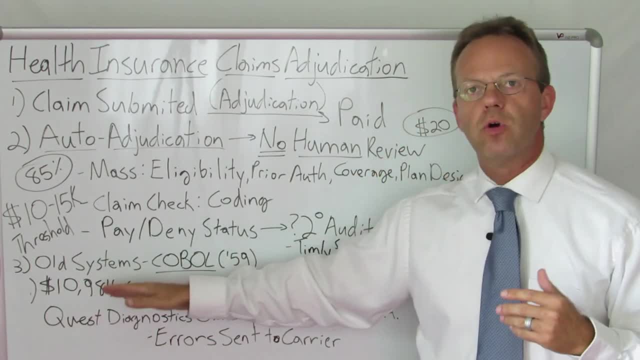 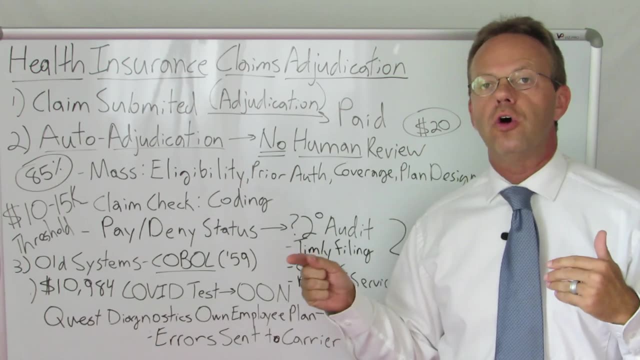 Where there was a $10,984 claim for a coronavirus, for a COVID test, right, A COVID test which in the article- and it was a COVID test for a pathologist himself, So it was a doctor himself who's familiar with the lab work itself. 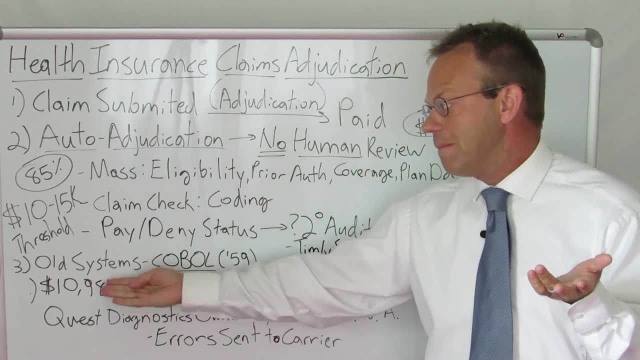 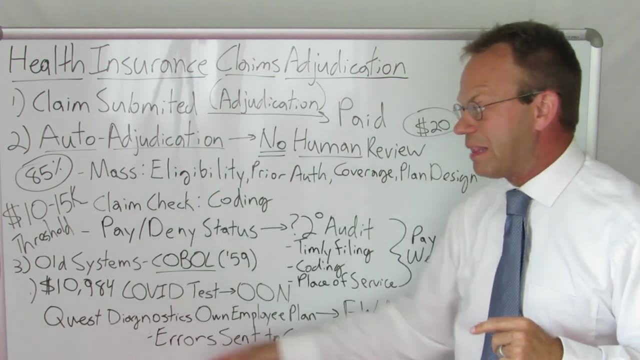 He's like it costs like $6 to do this test And they billed $10,984.. And guess what happened? The insurance company paid it. So, in other words, it made it through this entire process auto-adjudicated. 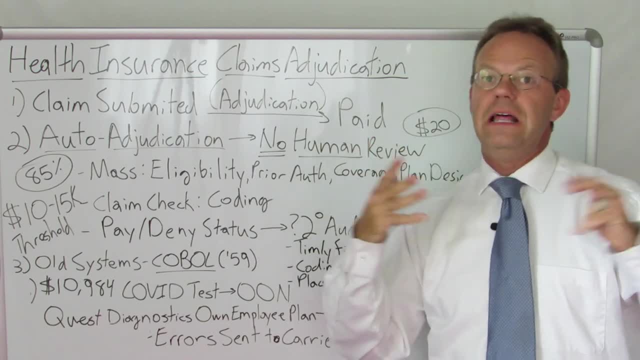 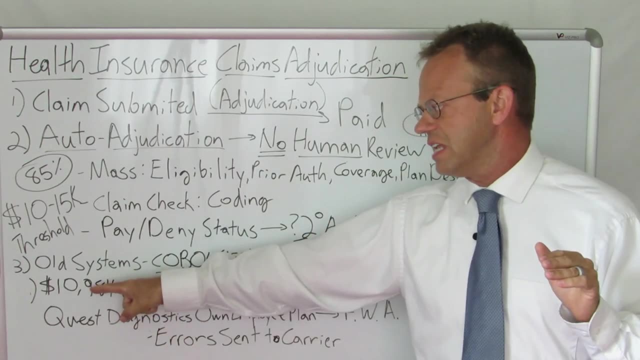 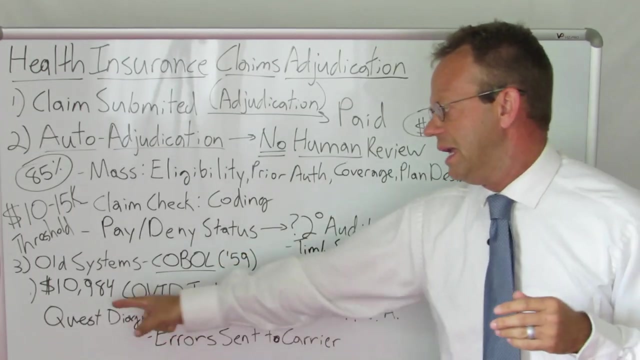 And it got paid Now and obviously that might be a problem If the out-of-network provider is billing $10,984 and is just getting paid. that makes you wonder, well, what else is getting through. Okay, Next up, Quest Diagnostics for their own employee health plan. had a physician running the health plan. 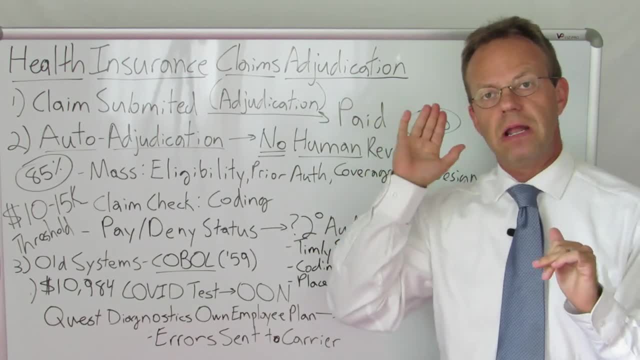 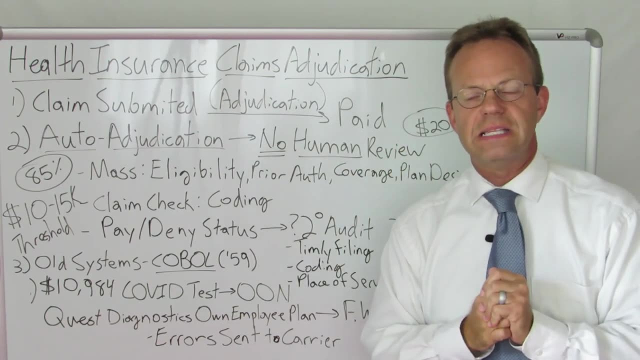 And I made a previous video about the Quest physician plan And it went from running 8% to 10% to being flat or even negative After they went through a whole bunch of reforms with their plan. One of the reforms that they did was they screened their own claims internally.